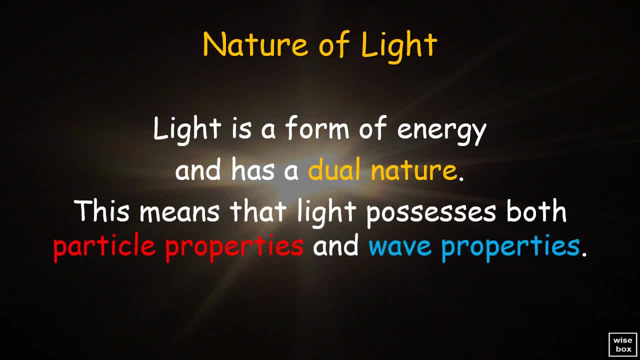 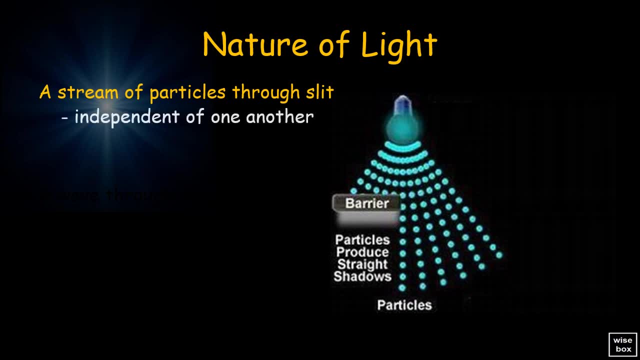 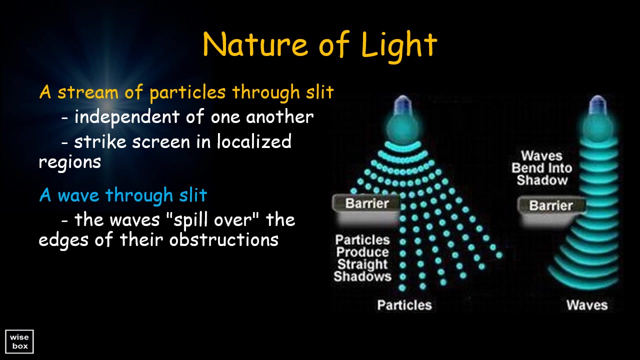 and wave properties. A stream of particles coming through each slit would come through independently of one another, striking the screen. in localized regions there are no fringe pattern and the particles produce straight shadows. when a wave passes through a slit or barrier, the waves spill over the edges of their obstructions. you can observe the waves bend into 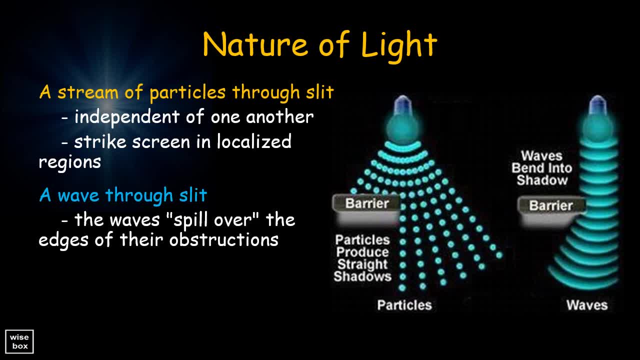 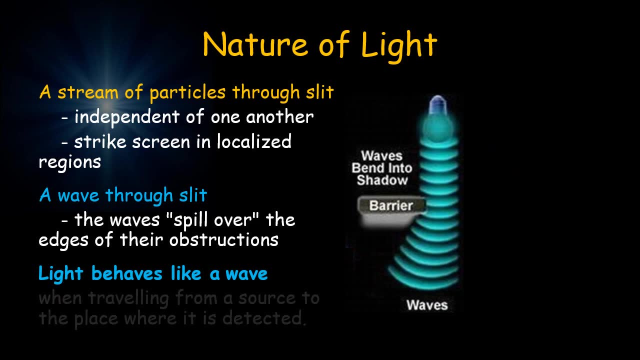 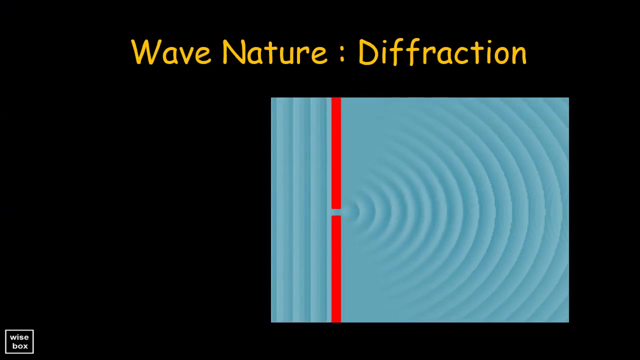 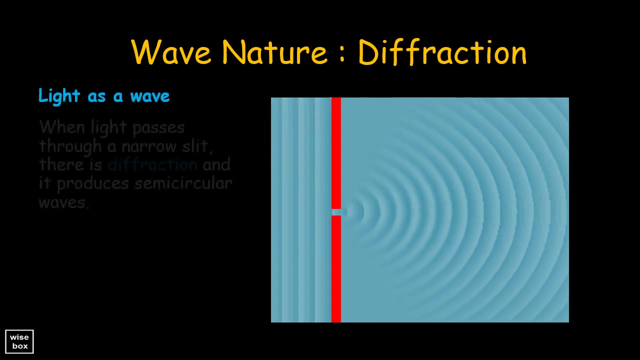 shadow, but through experiments it is observed that light behaves like a wave when traveling from a source to the place where it is detected. here is an illustration of the wave nature of light. when light passes through a narrow slit, there is diffraction and it produces semicircular waves. 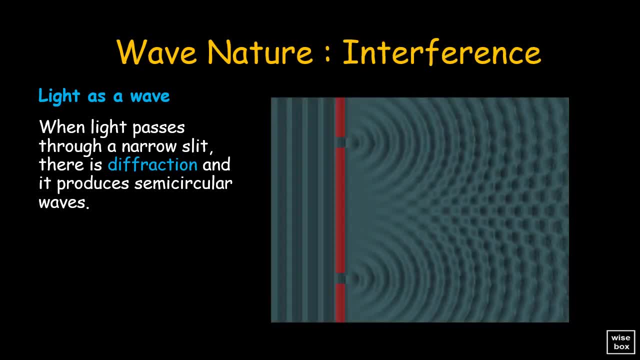 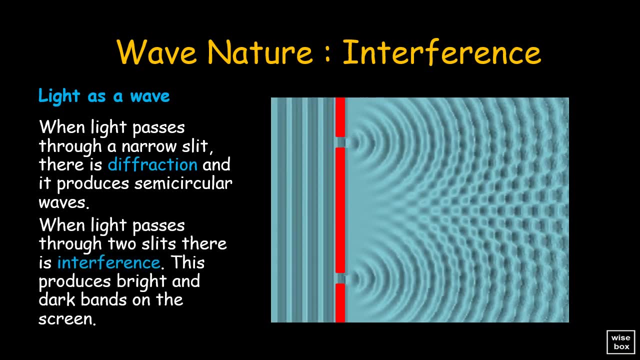 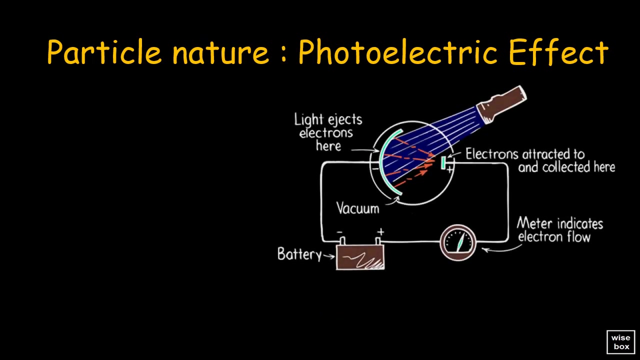 also, when the light waves passes through the two slits, there is interference and there is diffraction, producing bright and dark bands on the screen. this is a result that would not be expected if light consisted only of particles. here is an illustration showing the particle nature of light. 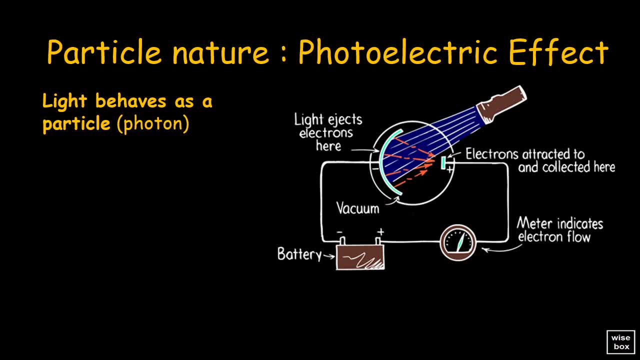 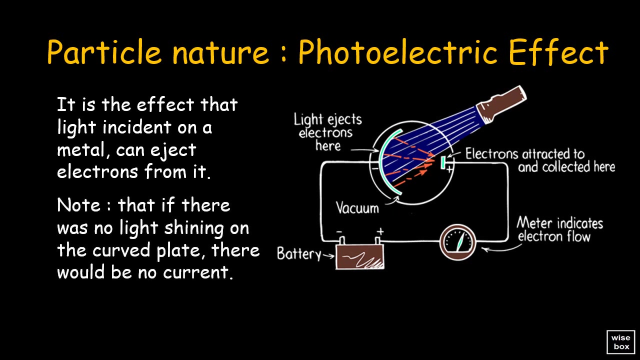 light behaves as a particle or photon when it is being emitted or when being absorbed at a detector. this is the photoelectric effect. it is the effect that light incident on a metal can eject electrons from it. note that if there was no light shining on the curved plate, there would be no current. 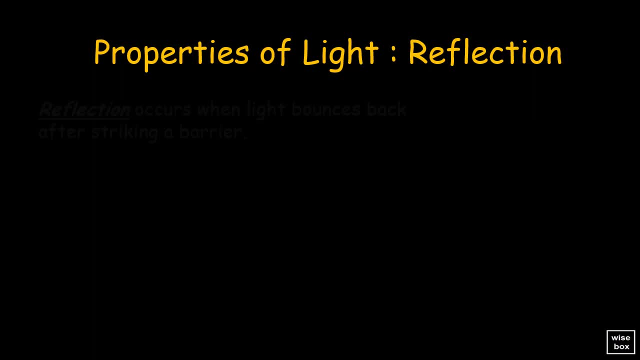 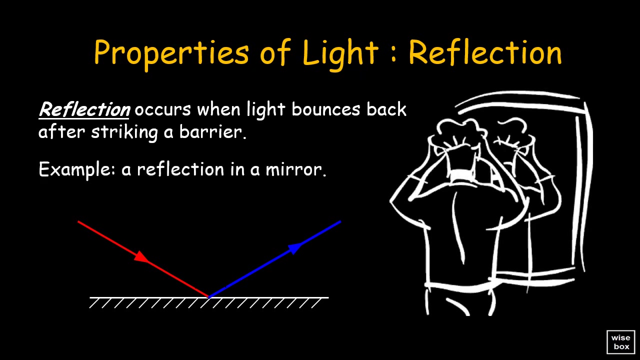 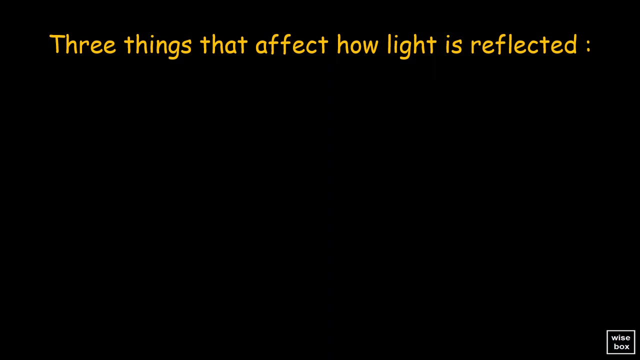 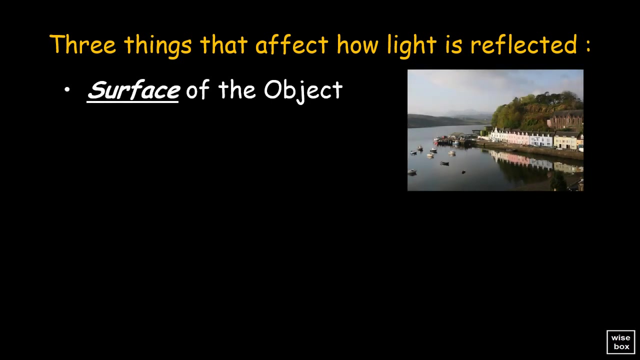 a property of light is reflection. reflection occurs when light bounces back after striking a barrier. this is an example of a reflection of light. one good example is reflection in a mirror. here are the three things that affect how light is reflected: the surface of the object. the colour of the object. 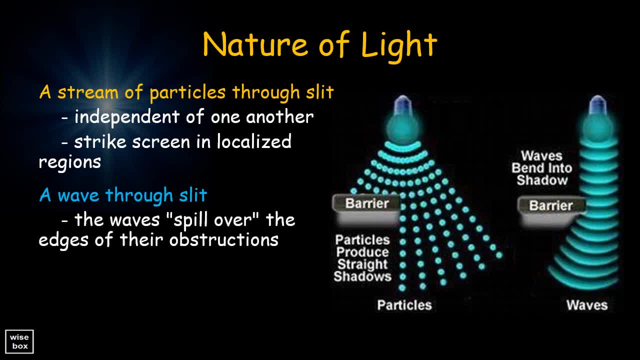 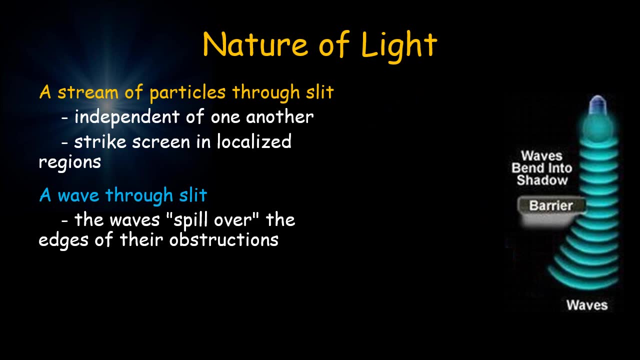 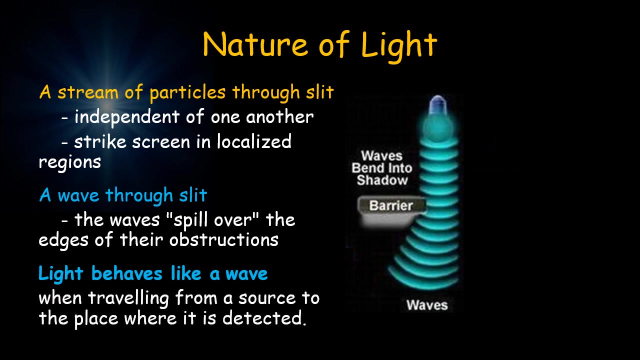 the waves spill over the edges of their obstructions. you can observe the waves bend into shadow, but through experiments it is observed that light behaves like a wave. when traveling from a source to the place where it is detected, the light is reflected in the area of the slit. 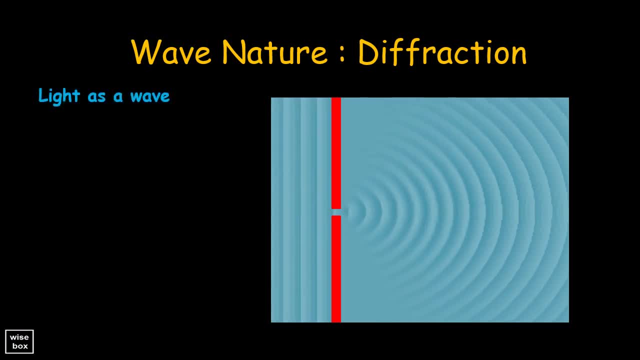 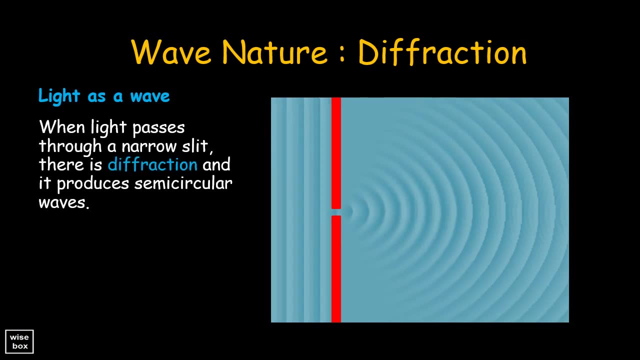 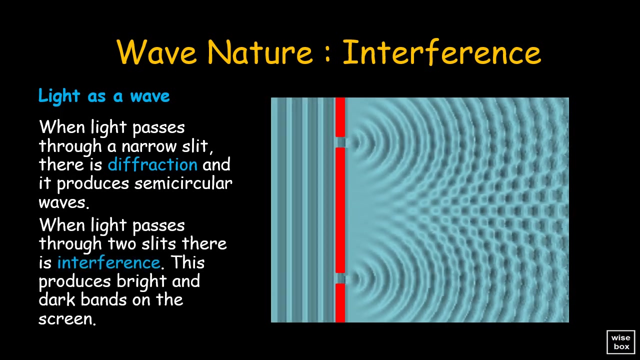 the light is reflected in the area of the slit. here is an illustration of the wave nature of light. when light passes through a narrow slit, there is diffraction and it produces semicircular waves. also, when the light waves passes through the two slits, there is interference. 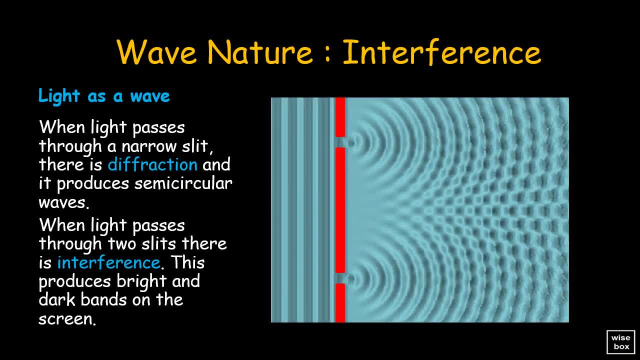 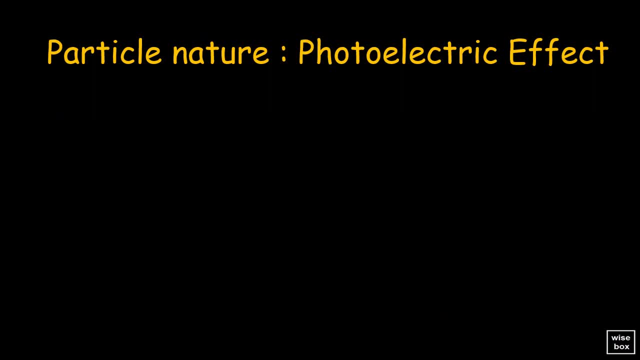 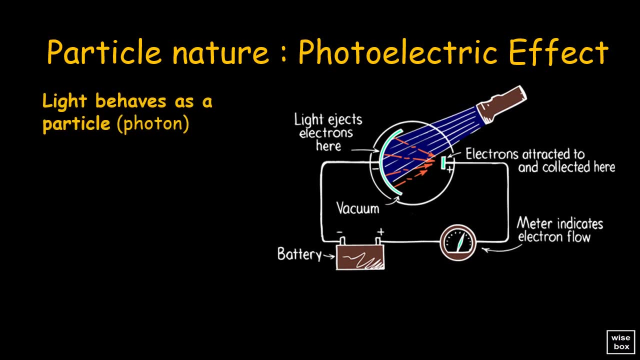 producing bright and dark bands on the screen. this is a result that would not be expected if light consisted only of particles. here is an illustration showing the particle nature of light. light behaves as a particle or photon when it is being emitted or when being absorbed at a detector. 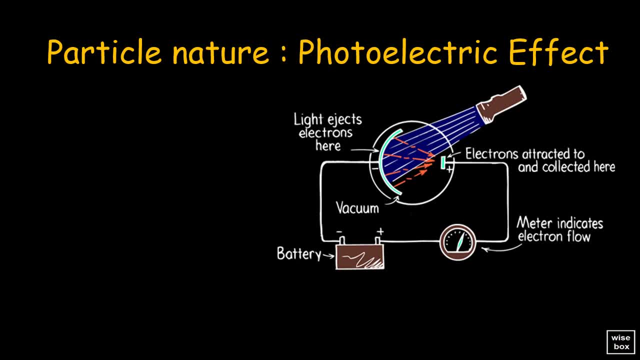 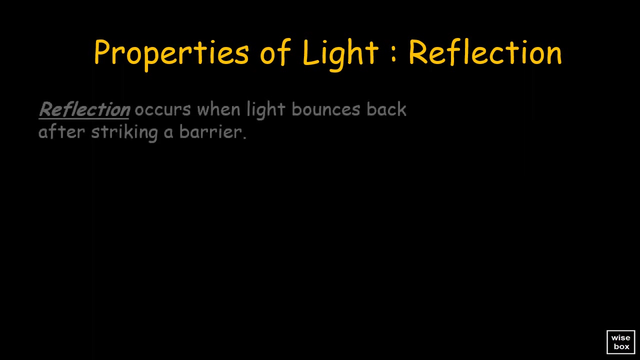 this is the photoelectric effect. it is the effect that light incident on a metal can eject electrons from it. note that if there was no light shining on the curved plate, there would be no current. a property of light is reflection. reflection occurs when light bounces back after striking a barrier. 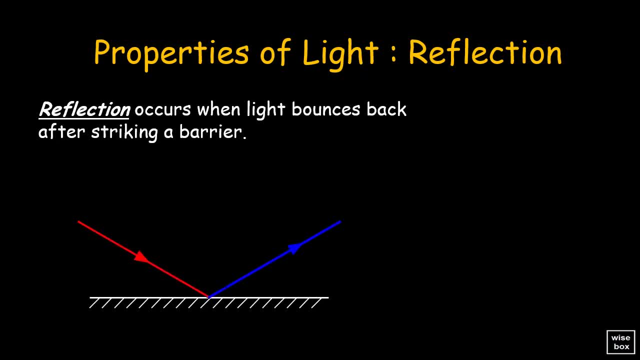 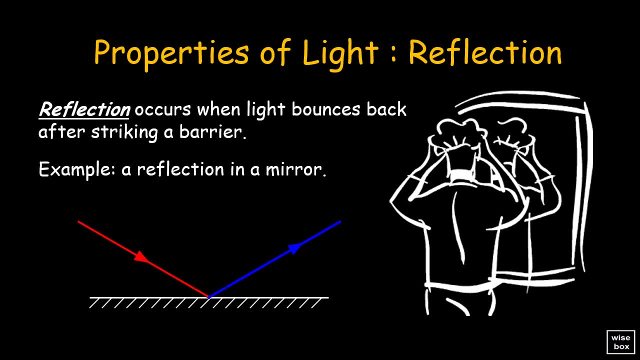 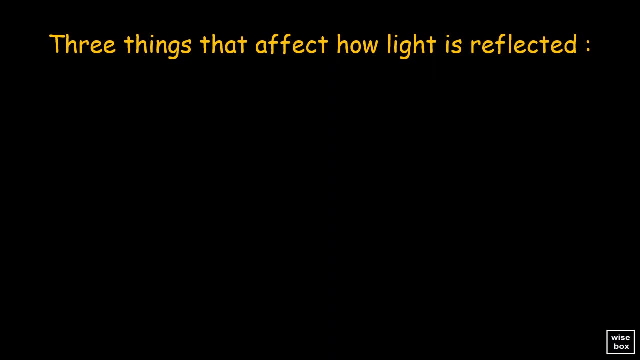 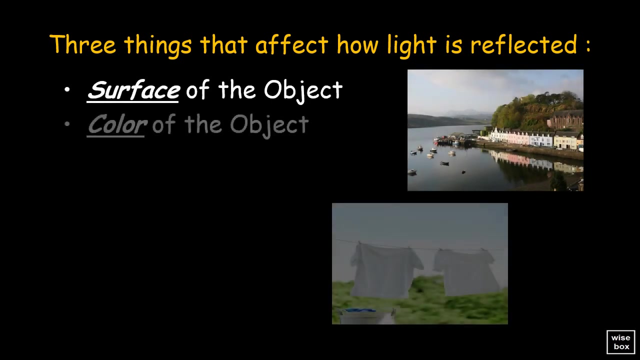 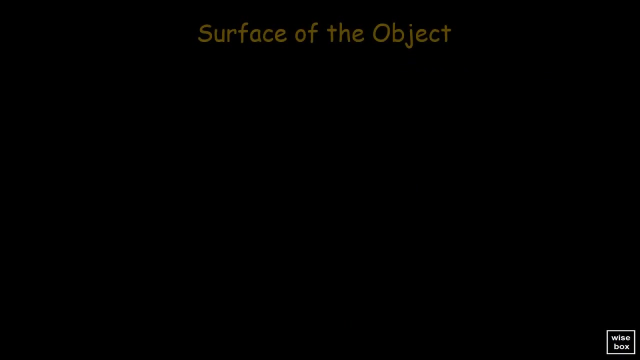 this will be reflected by lightrops. it is still a good plane later. one good example is reflection in a mirror. here are the three things that affect how light is reflected: the surface of the object, the color of the object and the shape of the object. Here is the effect of the surface of the object on how light is reflected. 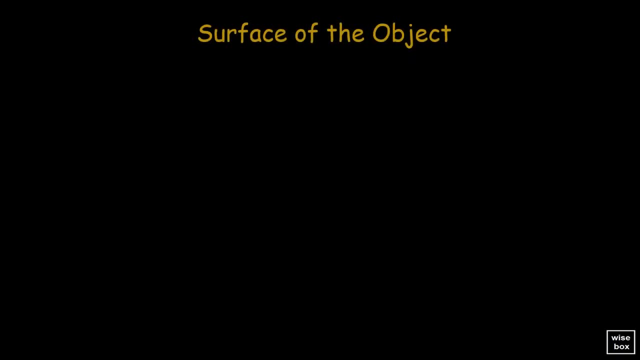 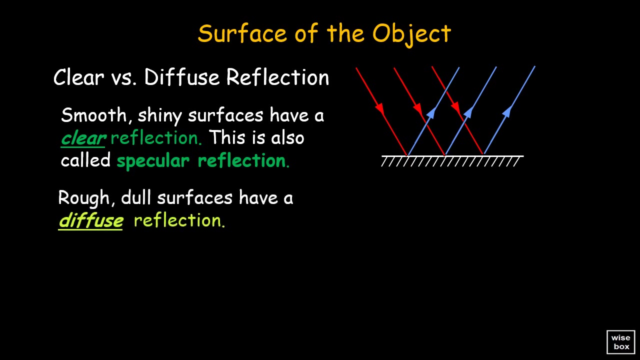 and the shape of the object. Here is the effect of the surface of the object on how light is reflected. Smooth, shiny surfaces have a clear reflection, And this is also called specular reflection, While rough, dull surfaces have a diffuse reflection. 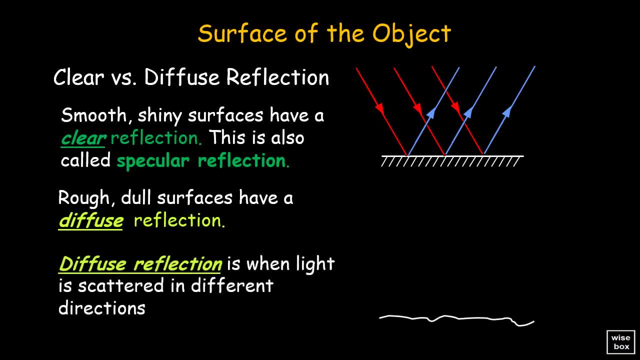 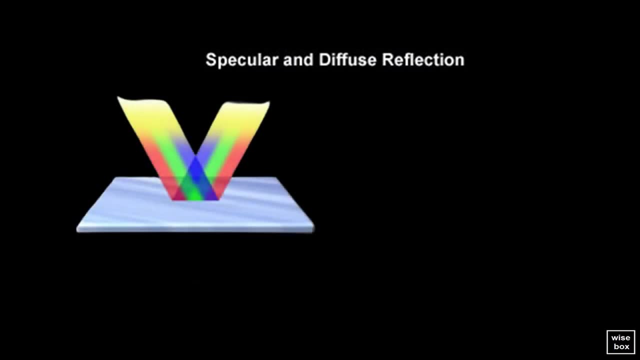 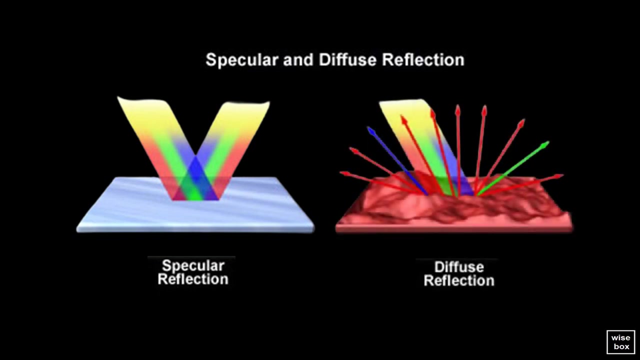 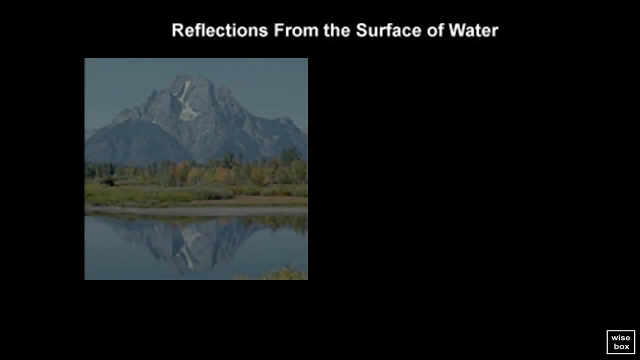 Diffuse reflection is when light is scattered in different directions. Here is specular reflection. The clear, smooth surface makes clear reflection, While the here is diffuse reflection. The rough surface scatters light in different directions. Here is an illustration of clear reflection. 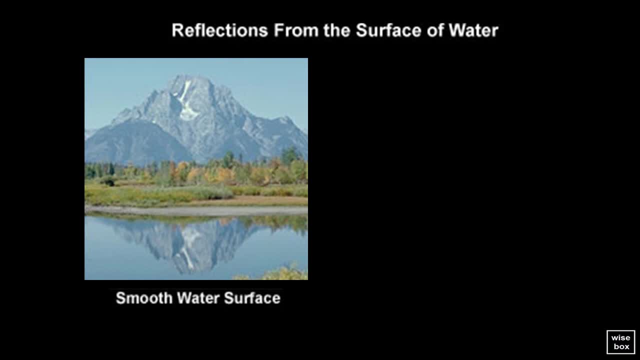 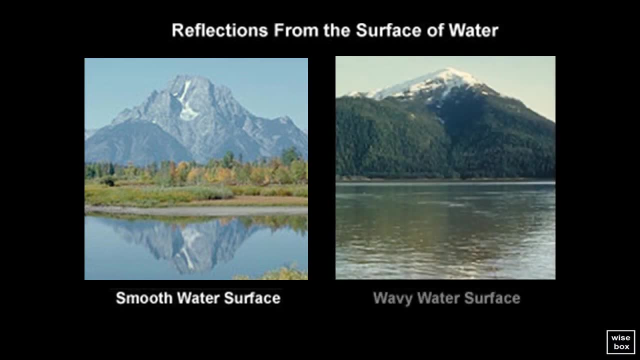 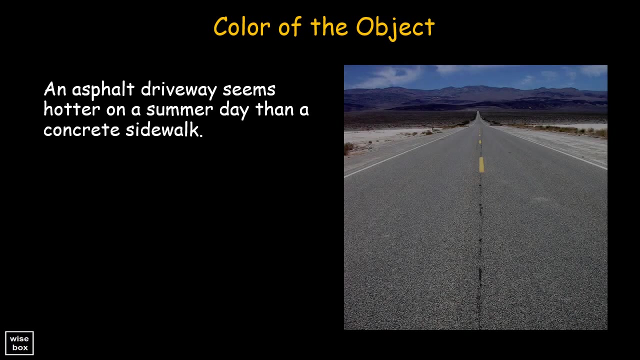 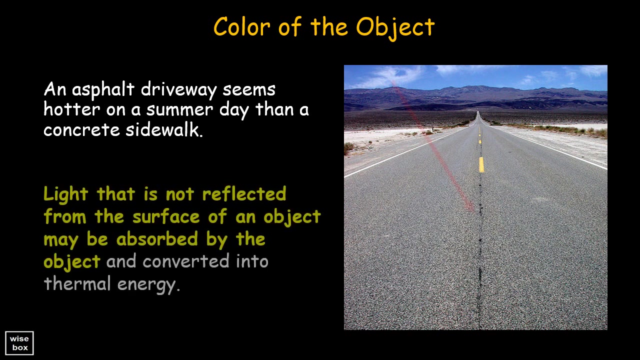 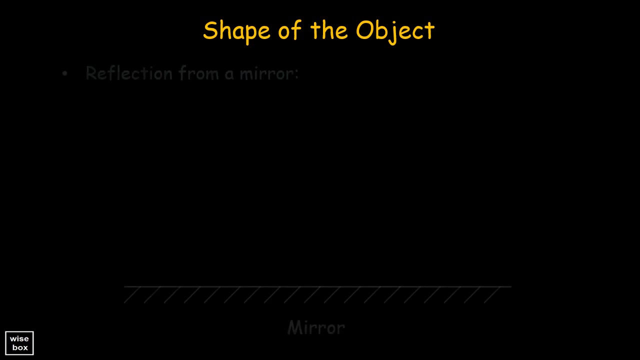 From a smooth water surface, While here is diffuse reflection From a wavy water surface. We can observe the free reflection of light from the surface. We can imagine what old earth looks like from an angle and line is the perpendicular line from the surface, then the reflected ray of light. 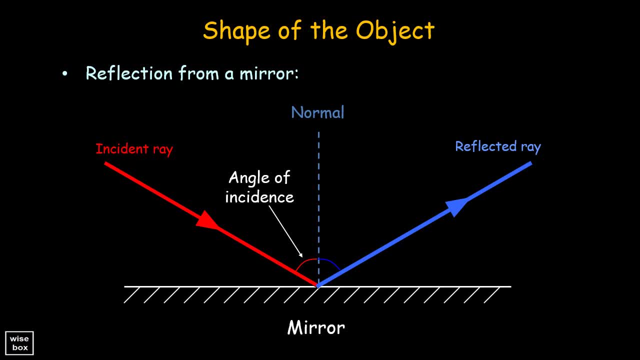 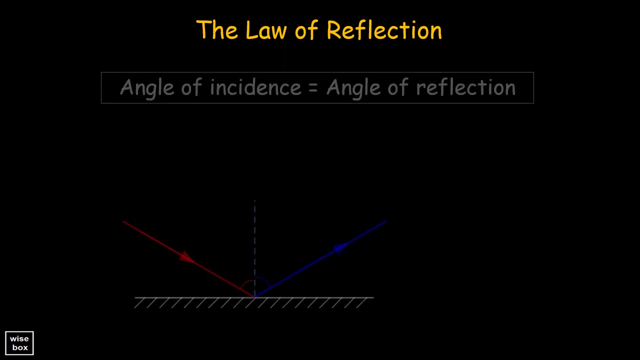 produced will in turn also have an angle of reflection measured from the normal line, light always reflects according to the law of reflection. the law of reflection states that the angle of incidence equals the angle of reflection. in other words, light gets reflected from a surface at the same angle that hits it. 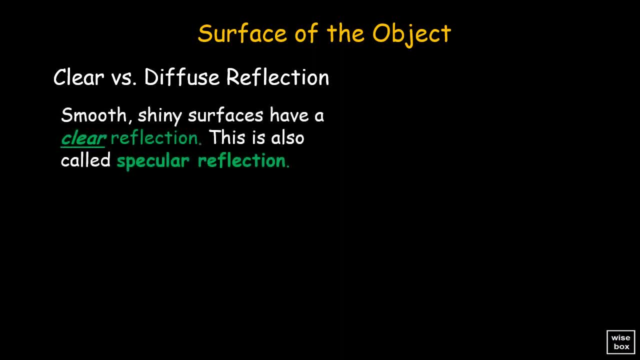 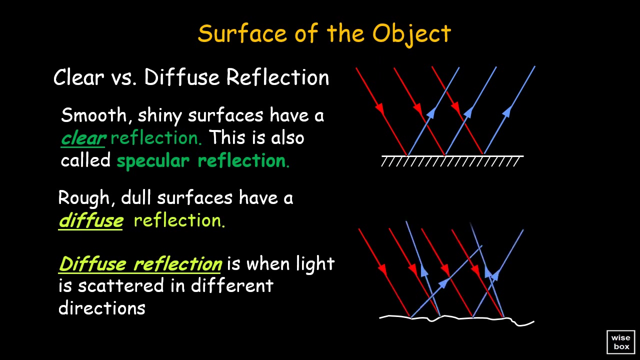 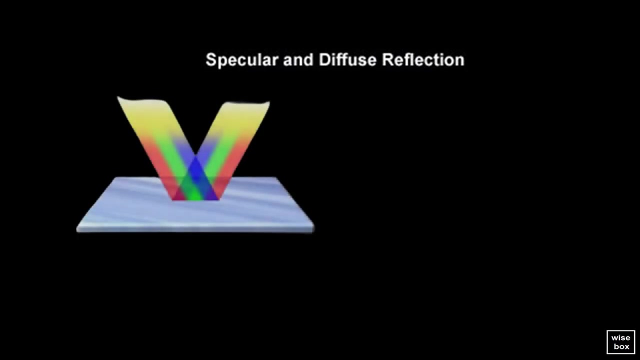 Smooth, shiny surfaces have a clear reflection, And this is also called specular reflection, While rough, dull surfaces have a diffuse reflection. Diffuse reflection is when light is scattered in different directions. Here is specular reflection. The clear, smooth surface makes clear reflection. 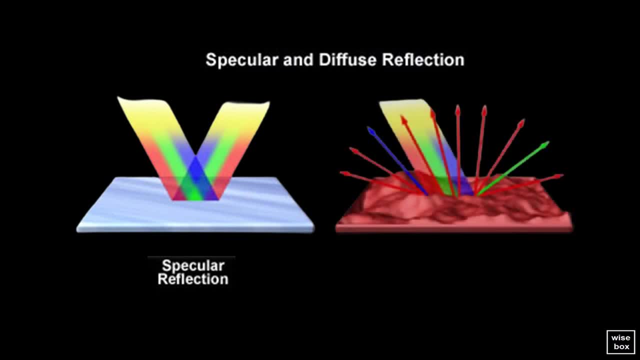 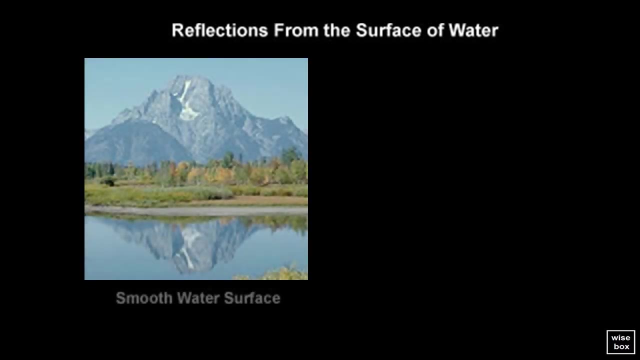 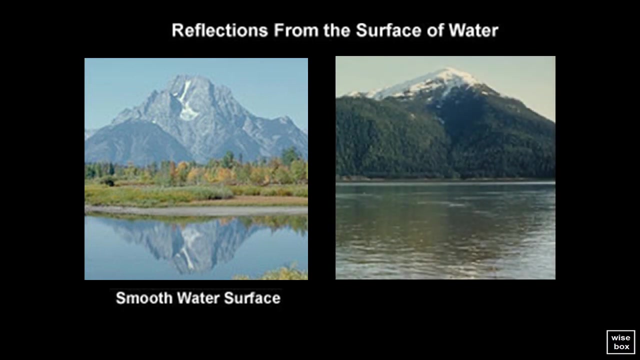 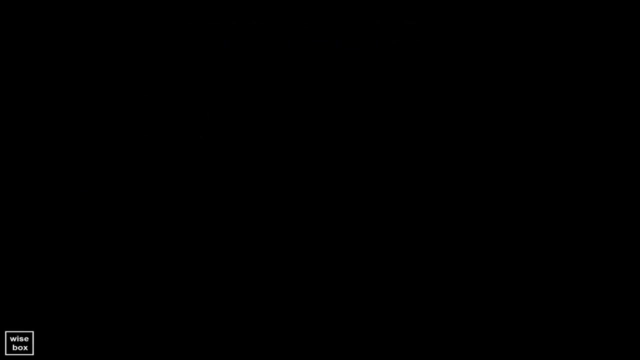 While the here is diffuse reflection, The rough surface scatters light in different directions. Here is an illustration of clear reflection From a smooth water surface, While here is diffuse reflection From a wavy water surface. Ever notice that an asphalt surface? 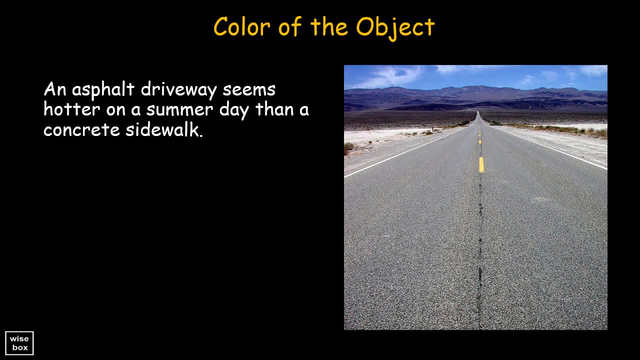 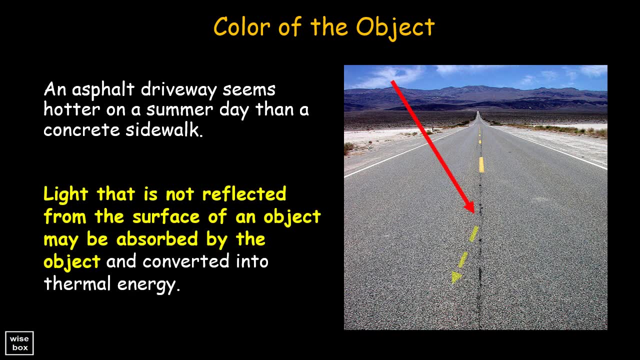 seems hotter on a summer day than a concrete sidewalk. This occurs because light that is not reflected from the surface of an object may be absorbed by the object and converted into thermal energy. To see how the shape affects the reflection of light. 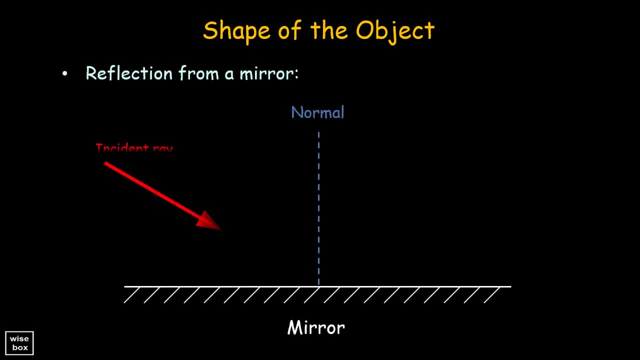 let's look at reflection from a mirror. An incident ray of light will form an incident angle from the normal line. This normal line is the perpendicular line from the surface. Then the reflected ray of light produced will in turn also have an angle of reflection measured from the normal line. 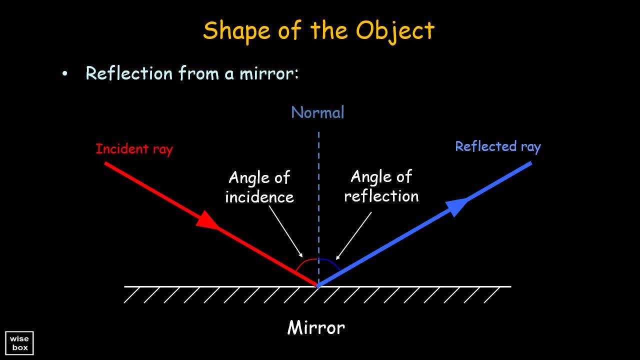 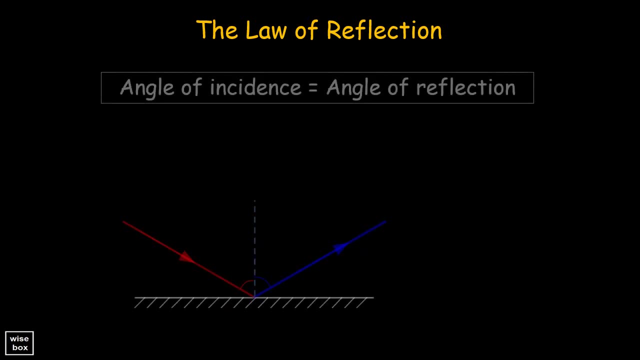 The angle of reflection is measured from the normal line. The angle of reflection is measured from the normal line. The angle of reflection is measured from the normal line. Light always reflects according to the law of reflection. The law of reflection states that the angle of incidence equals the angle of reflection. 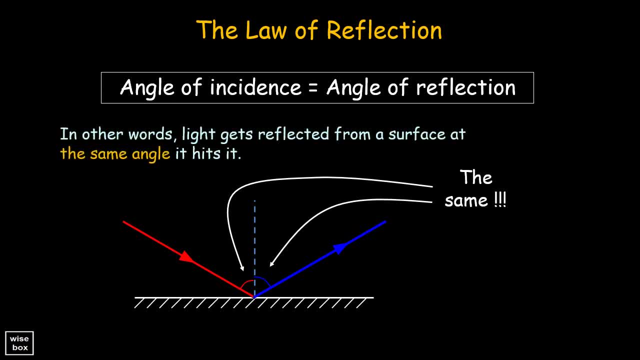 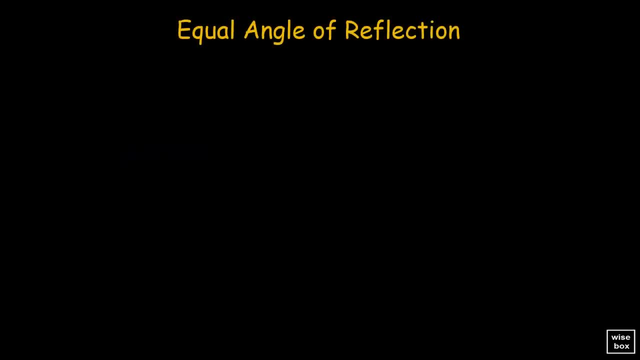 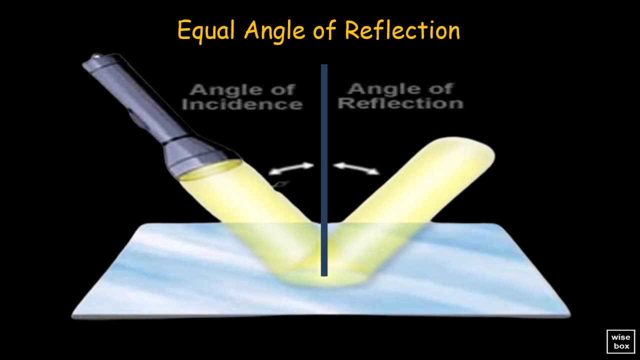 In other words, light gets reflected from a surface at the same angle it hits it. This illustration shows that the light from an ordinary flashlight follows the law of reflection when its light hits a reflective surface like a mirror. There are typically three types of mirrors. 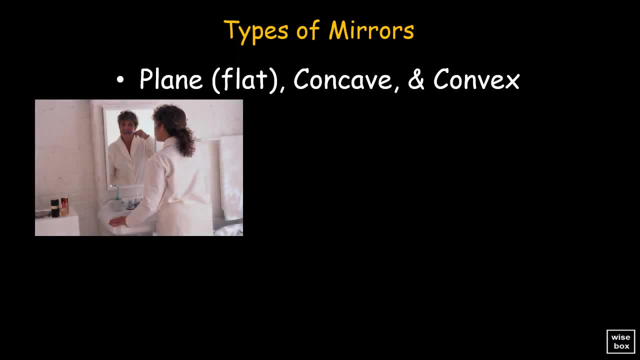 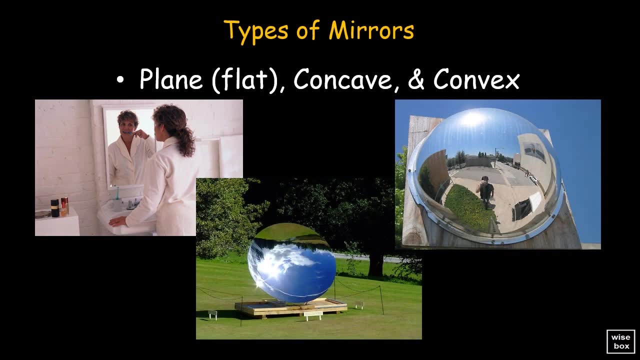 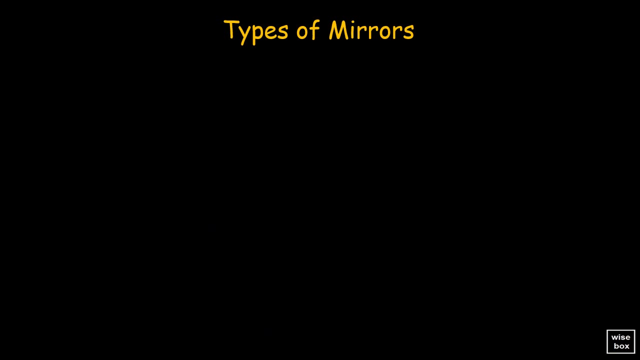 The plain or flat mirror, The concave mirror And the convex mirror. First we have the plain mirror. It has a flat surface. In here, light is reflected straight back, Resulting in an upright image that is the same size as the original object. 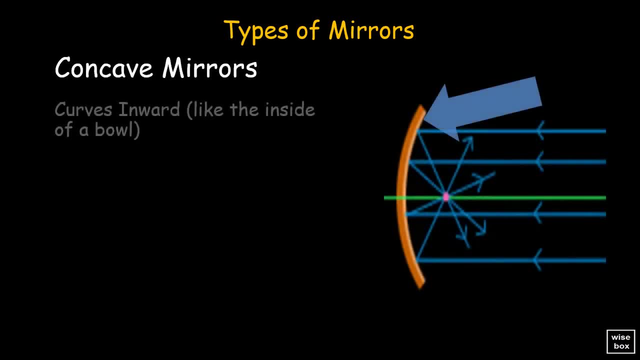 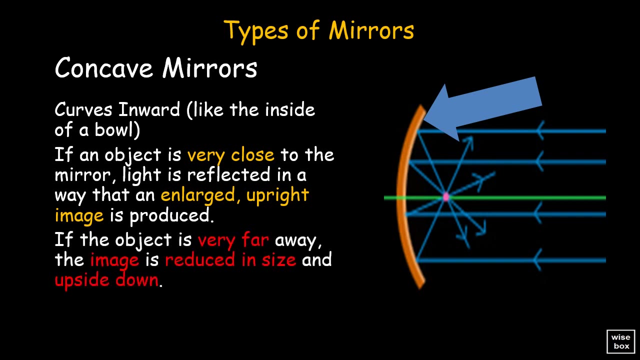 Concave mirrors are curved inward, like the inside of a bowl. If an object is very close to the mirror, light is reflected in a way that an enlarged upright image is produced. If the object is very far away, the image is reduced in size and upside down. 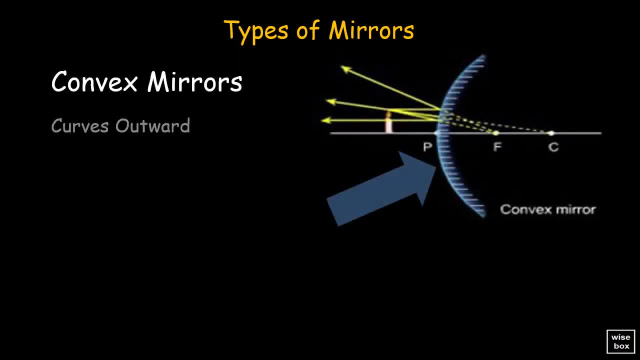 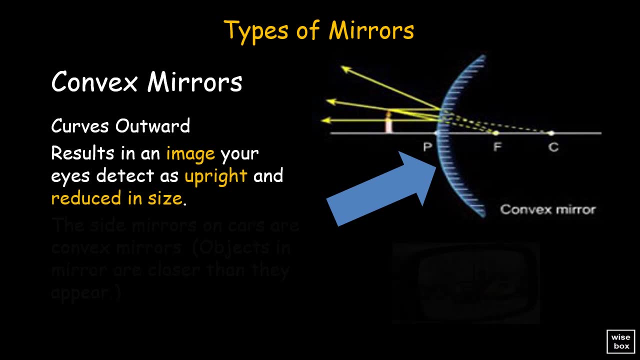 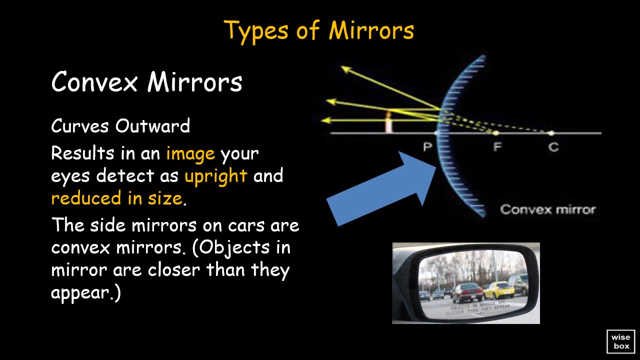 Concave mirrors are curved outward. This results in an image your eyes detect as upright and reduced in size. The side mirrors on cars are convex mirrors. Objects in mirror are closer than they appear. Here are examples of images in convex and concave mirrors. 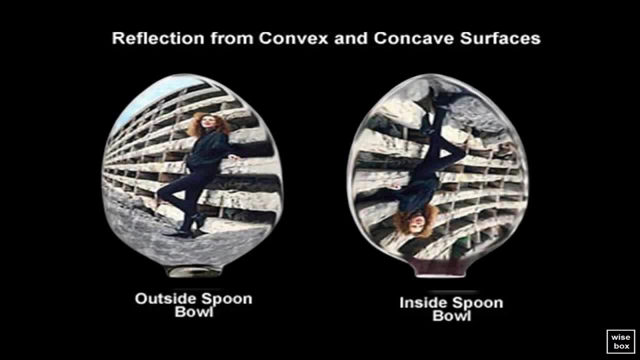 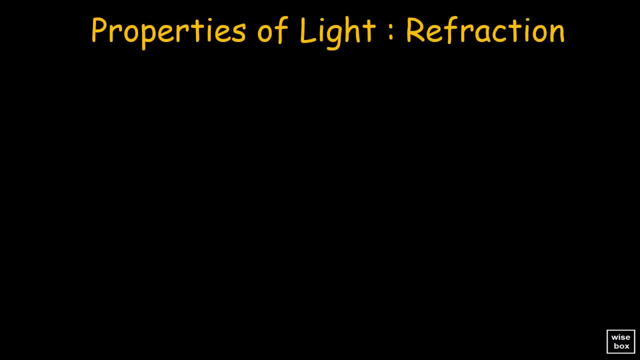 The upright image from the convex surface of outside spoon bowl. The inverted image from the concave surface of inside spoon bowl. Another property of light is refraction. It is the bending of a light as it passes from one medium to another. 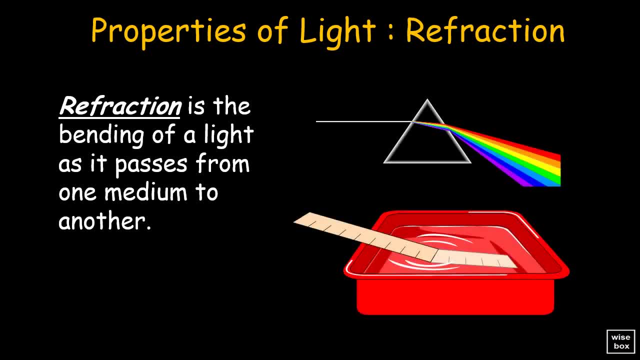 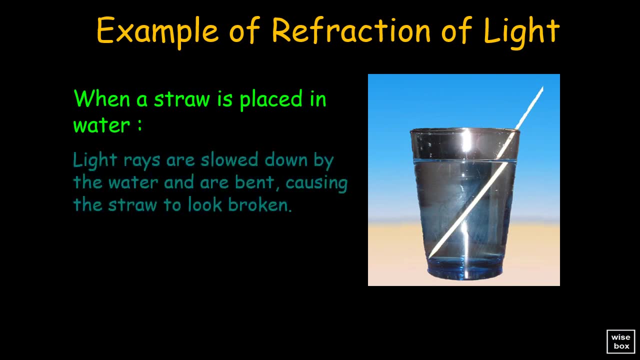 This phenomena happens when light passes through substances with different densities, Its speed changes and therefore it bends. When a straw is placed in water, it looks like this In this case: the light rays are slowed down by the water and are bent, causing the straw to look broken. 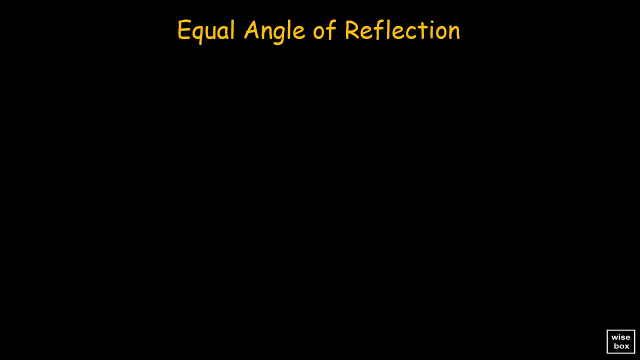 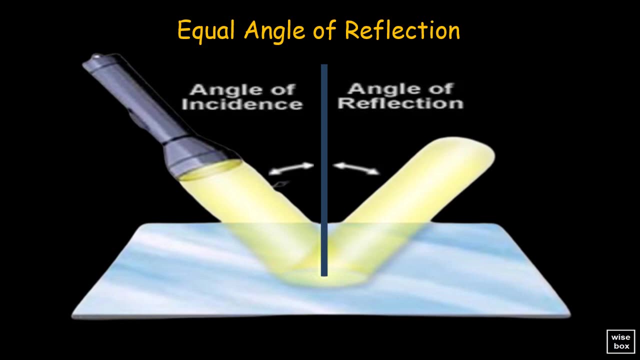 this is the angle of incidence that a reflection is at and, as we can see, the light always reflects on a surface at the same angle it hits it. this is the. This illustration shows that the light from an ordinary flashlight follows the law of reflection when its light hits a reflective surface like a mirror. 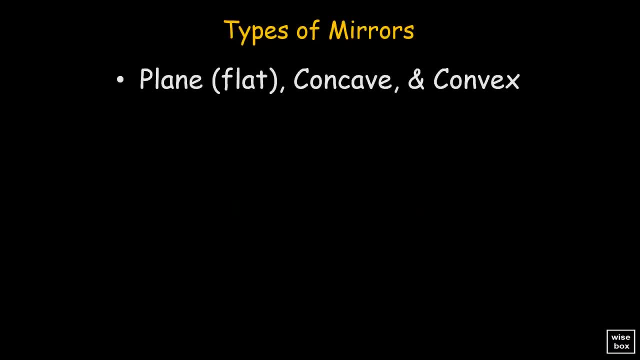 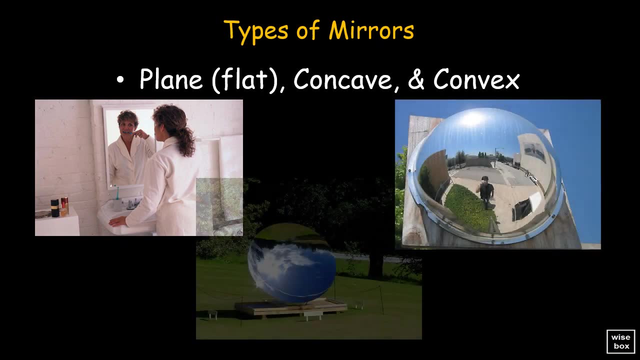 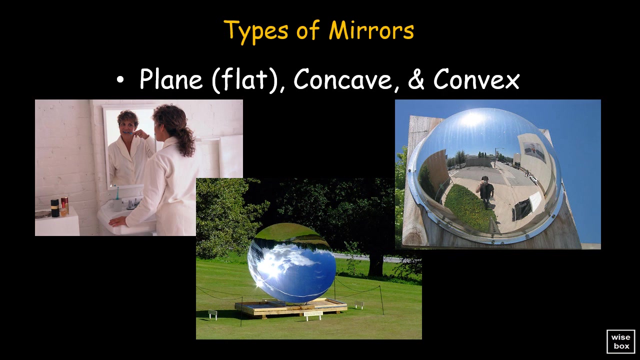 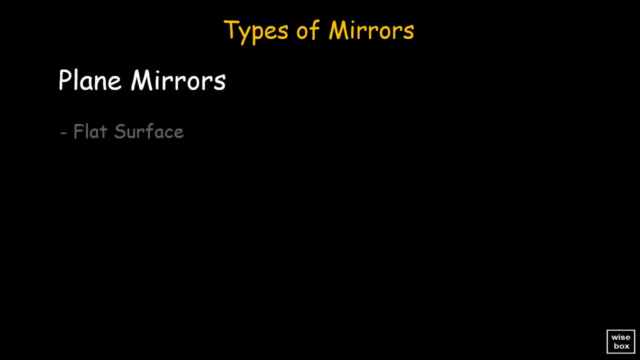 There are typically three types of mirrors: The plain or flat mirror, The concave mirror And the convex mirror. First we have the plain mirror. It has a flat surface. In here, light is reflected straight back, resulting in an upright image. that is the. 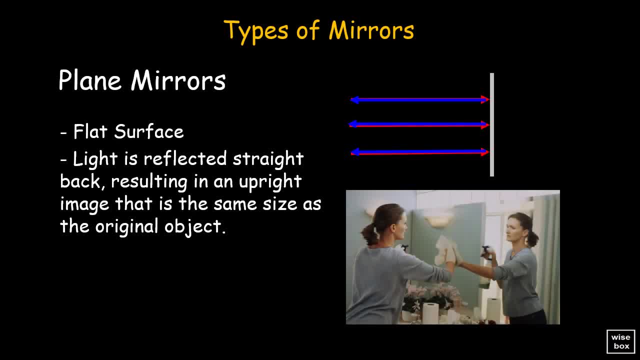 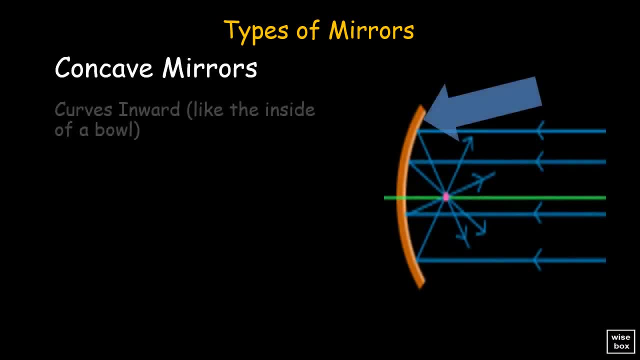 same size as the original object. Next we have the flat mirror. Concave mirrors are curved inward like the inside of a bowl. If an object is very close to the mirror, light is reflected in a way that an enlarged upright image is produced. 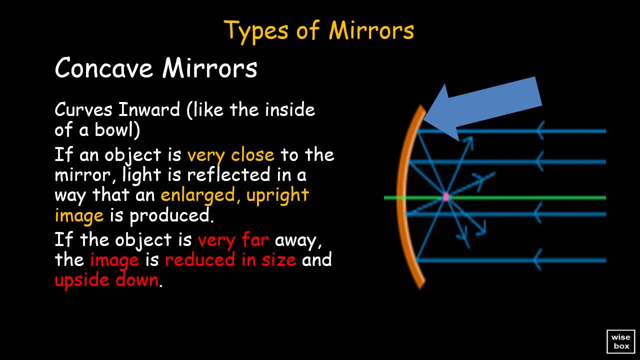 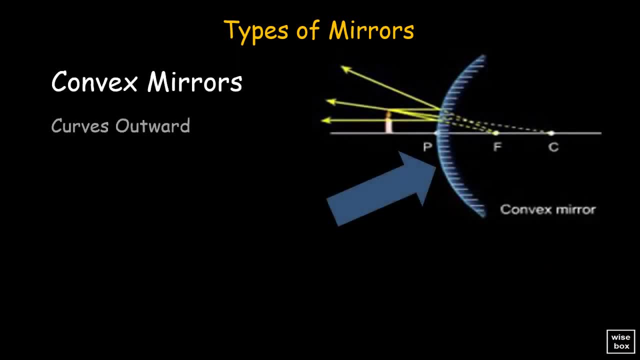 If the object is very far away, the image is reduced in size and, upside down, Concave mirrors are curved outward. This results in an image your eyes detect as upright Concave mirrors are curved outward. This results in an image your eyes detect as upright. 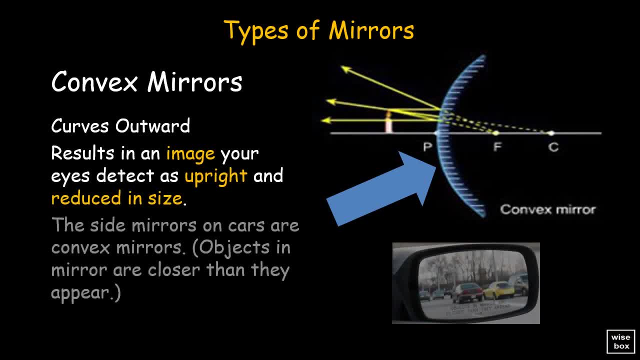 And reduced in size. The side mirrors on cars are convex mirrors. Objects in mirror are closer than they appear. The side mirrors on cars are convex mirrors. Objects in mirror are closer than they appear. Here are examples of images in convex and concave mirrors. 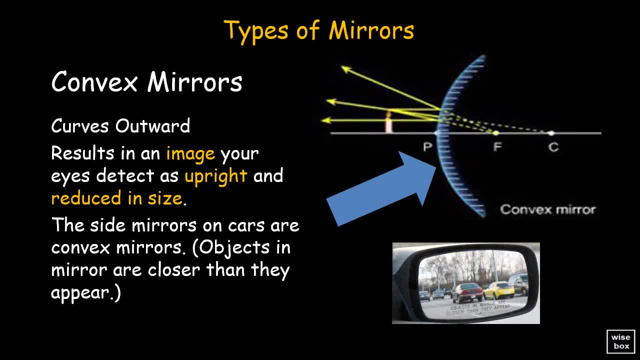 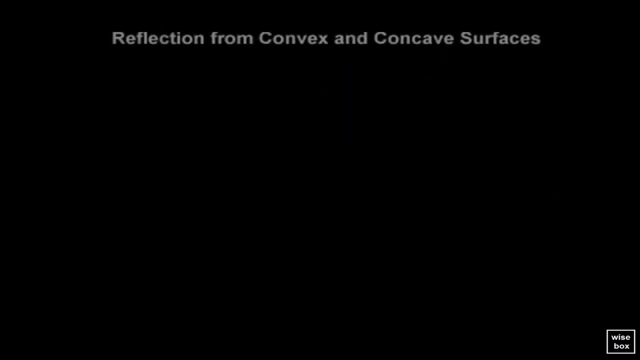 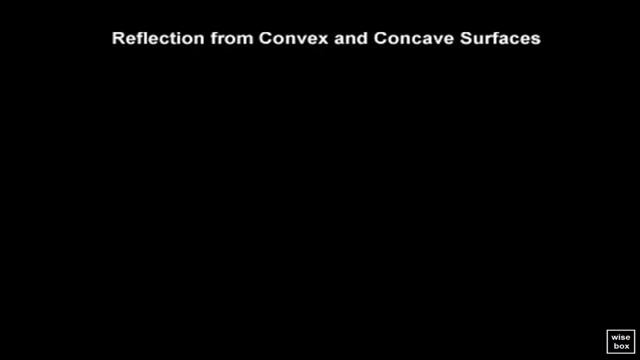 The inverted image from the concave surface of inside spoon bowl. The upright image from the convex surface of outside spoon bowl. The inverted image from the concave surface of inside spoon bowl. The upright image from the convex surface of outside spoon bowl. 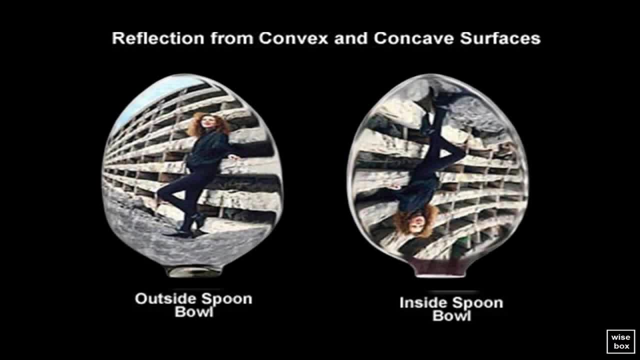 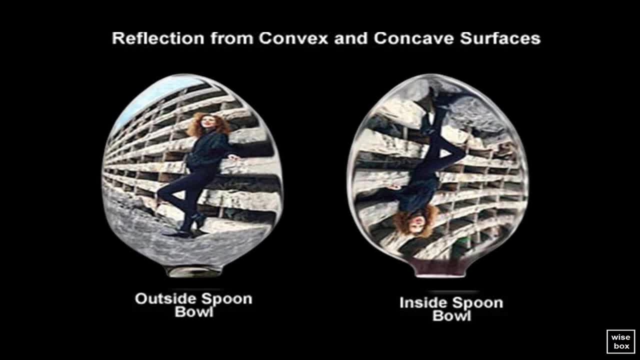 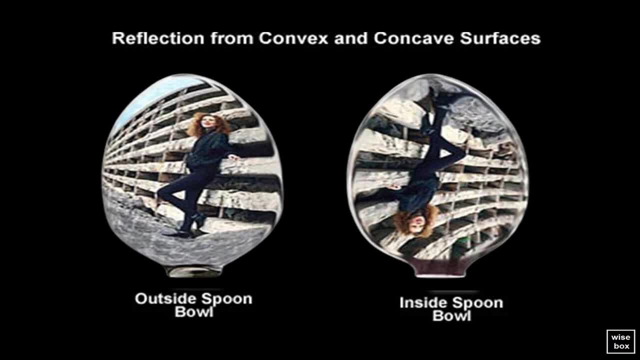 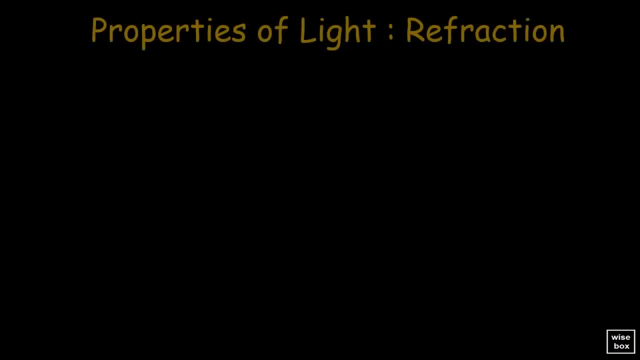 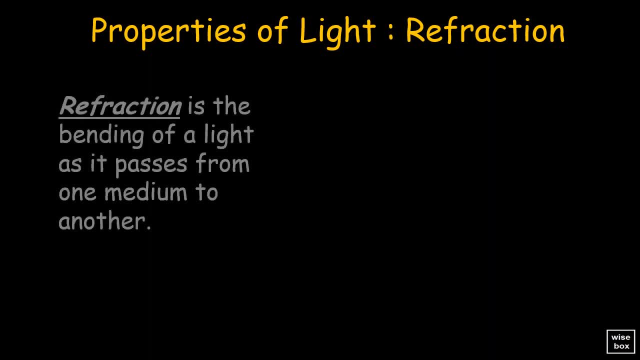 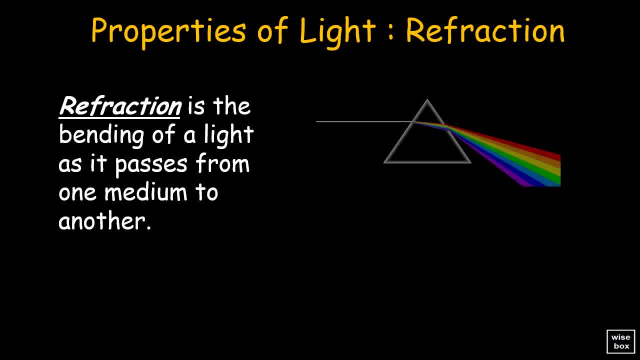 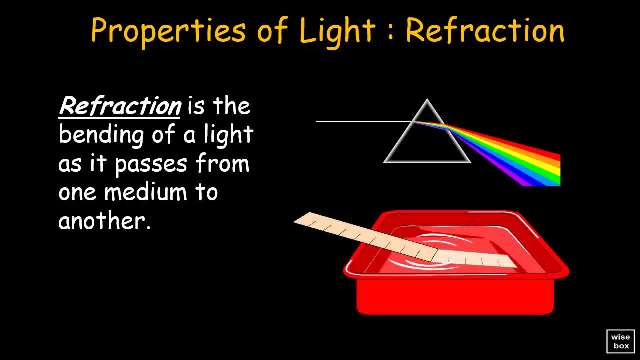 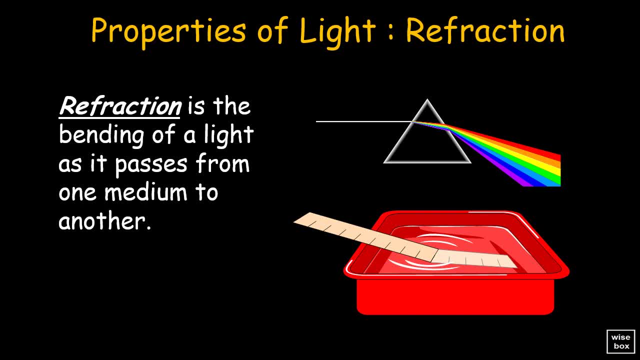 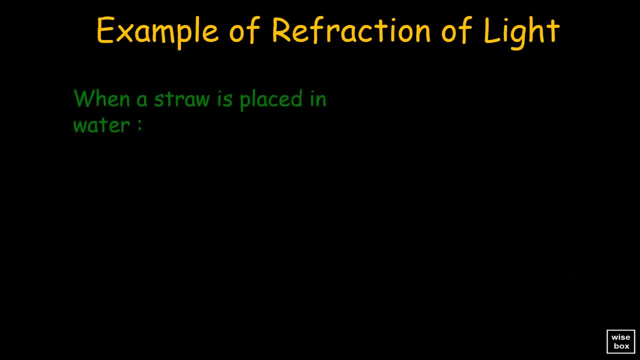 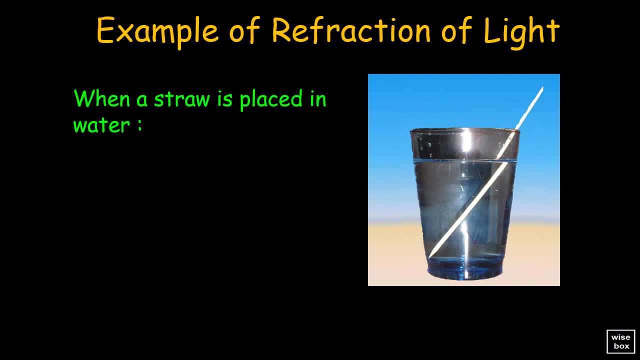 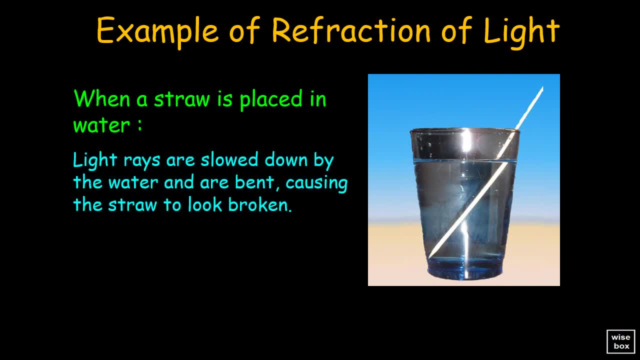 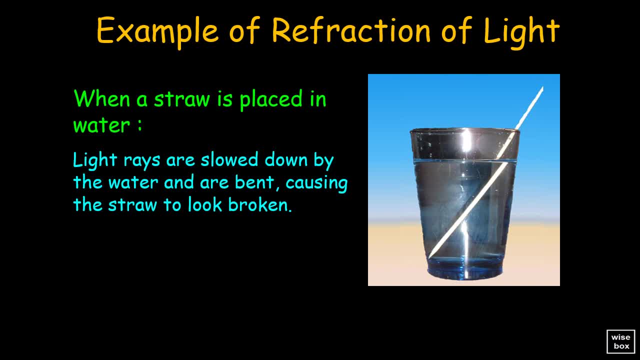 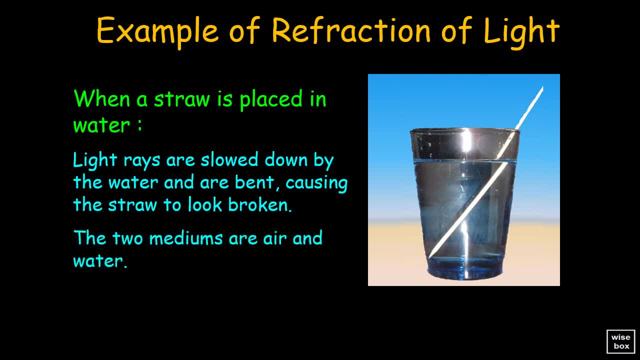 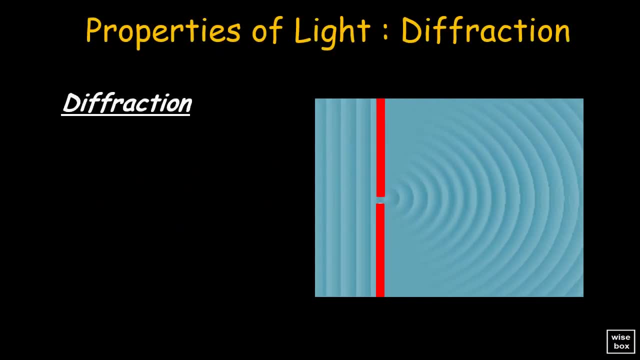 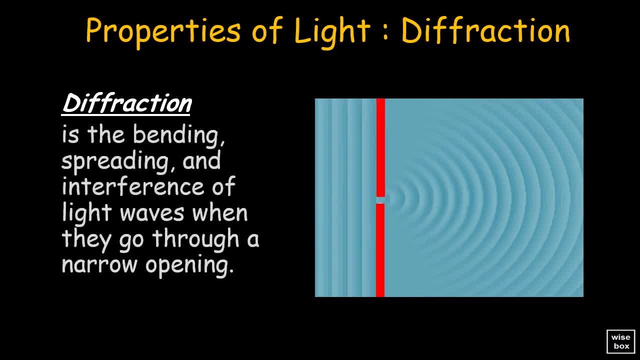 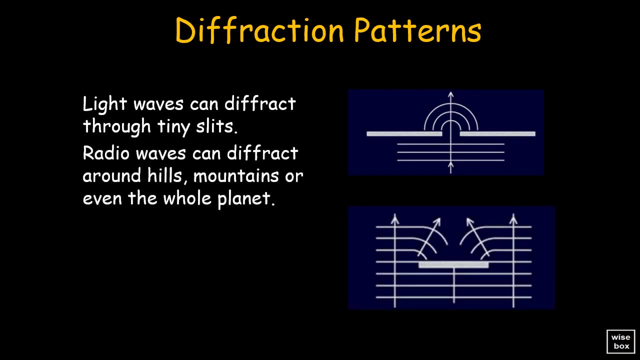 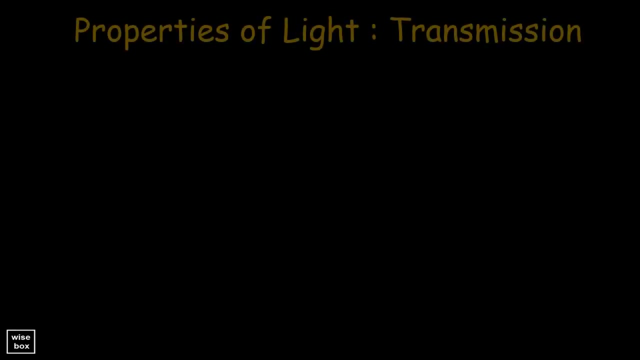 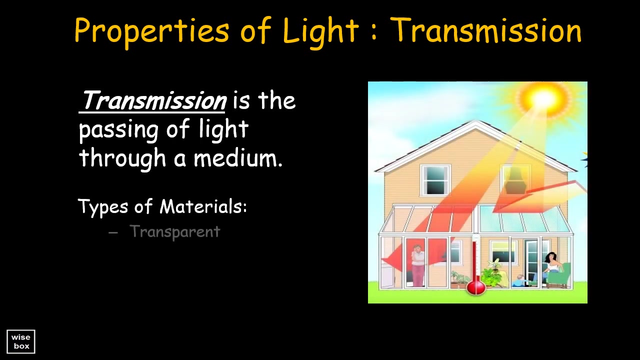 opening. light waves can diffract through tiny slits. radio waves can diffract around hills, mountains or even the whole planet. x-rays can diffract around atoms. transmission is the passing of light through a medium. transparent materials allows all light to pass through. translucent materials allows only some.